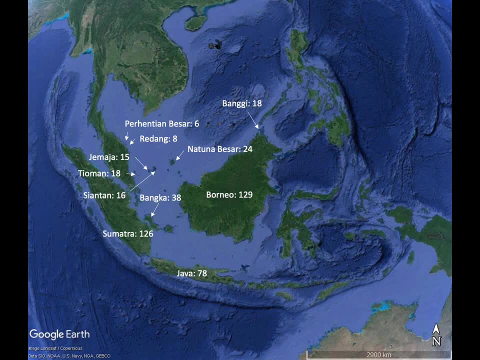 then climate will play a role. But what does it do With harsher climates limiting the number of species that can occur on an island? because only species with adaptations to survive harsh conditions can survive there. Similar islands, but in milder climates, would likely have higher species richness. 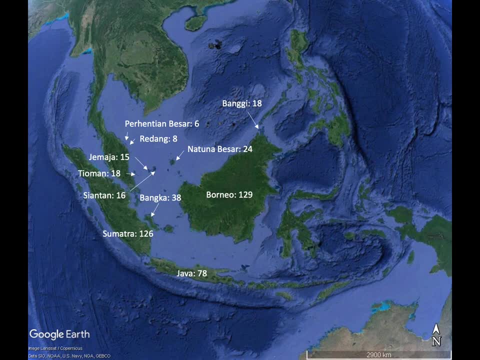 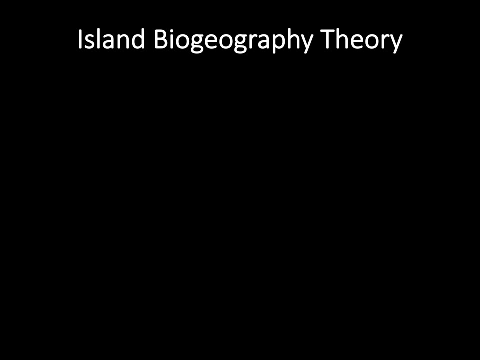 since more species can cope with the conditions on those islands. But within a single group of islands that share roughly the same climate, other factors must be driving variation. This is exactly the question that grabbed the attention of two ecologists, EO Wilson and Robert MacArthur. 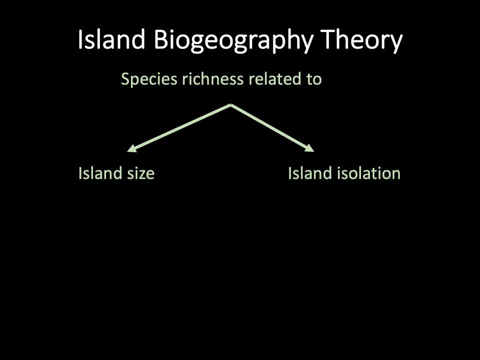 They theorized that the size and the isolation of islands would strongly determine how many species occur on those islands, Particularly through the effect of island size and island isolation on the colonization and extinction rate of species on those islands. Their ideas were formalized as the equilibrium theory of island biogeography. 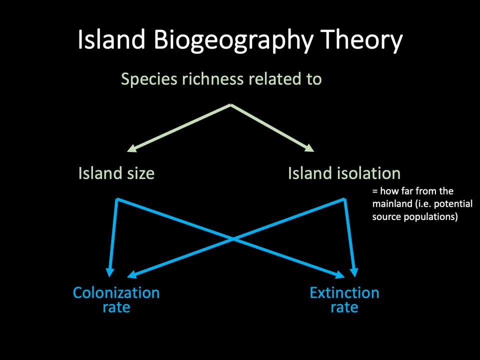 Just to be clear here: isolation refers to how far an island is from an area where species could colonize the island from. We typically say isolation reflects the distance between an island and the mainland area where all the species that potentially could colonize that island are. 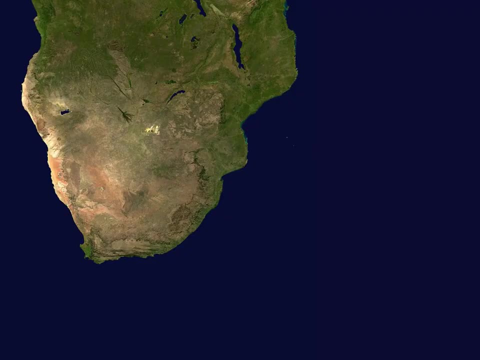 To understand this theory, let's imagine a scenario of a new oceanic island formed by an undersea volcano. This island is formed near a large, previously existing habitat, what we'd call the mainland. Due to natural dispersal, we'd expect that plants from the mainland would eventually arrive at the island and establish there. 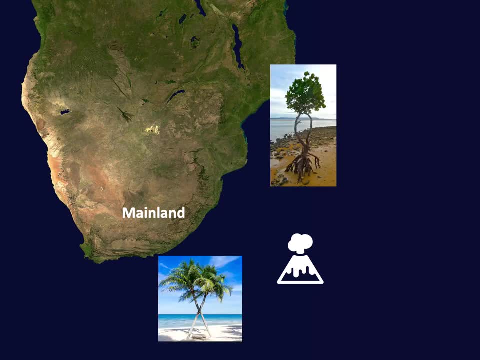 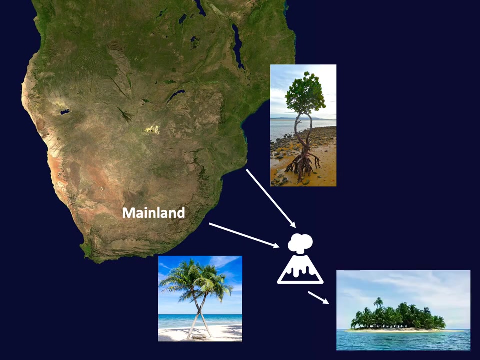 For example, we'd have species of mangrove trees and palms that occur along the southern African coast dispersing to the new island on ocean currents And then, through time, we'd expect to see more and more species arriving at the island, until we have an island with a roughly stable number of species occurring on it. Okay, let's go a little deeper into this now, thinking specifically about colonization and extinction rates and how they will change through time. In other words, how will colonization and extinction rates differ between islands soon after the island was formed compared to many years later? 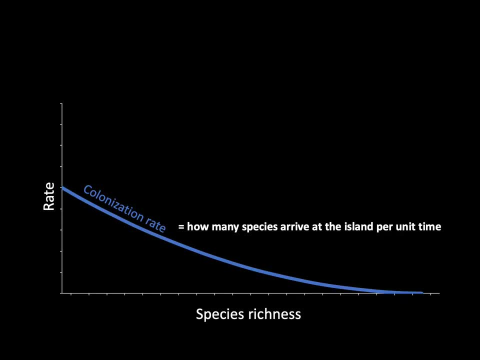 when lots of species already occur on it. So on this graph we've got the rate of colonization shown in blue and that's plotted against species richness. So we would expect that species from the mainland would gradually colonize the new island. 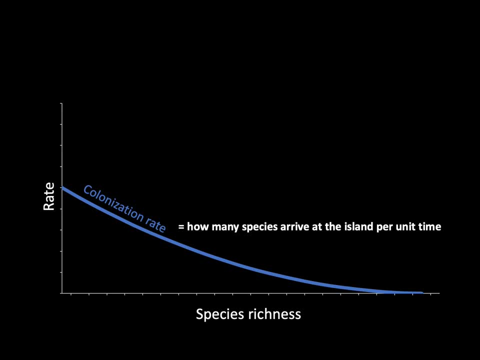 with this colonization rate declining as more and more species colonize the island. Now, this would occur simply because there are then less species on the mainland that haven't yet colonized the island as we get more and more of those mainland species colonizing the island. 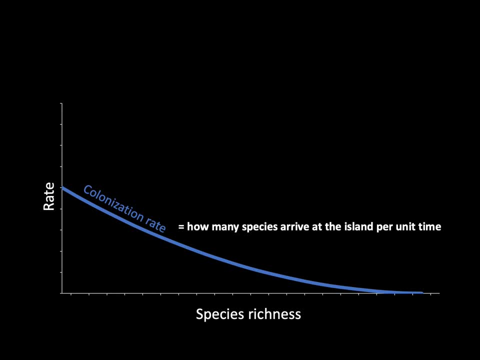 So, for example, at the beginning, every species that arrives at the island is a new species for the island. However, later on, when many species are already on the island, when an organism then arrives at the island, the chances are high. 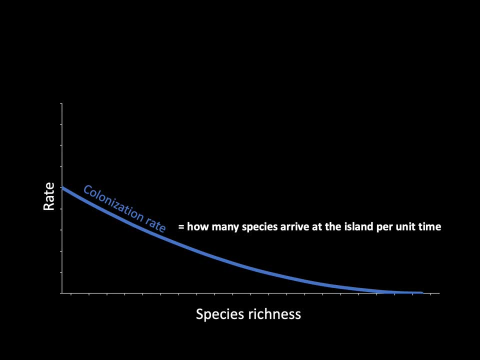 that other members of its species are already there and therefore colonization rate decreases as species richness increases. In other words, we can imagine a new island. when there are no species on the island, the island will experience a high colonization rate, since any species that successfully disperse to the island 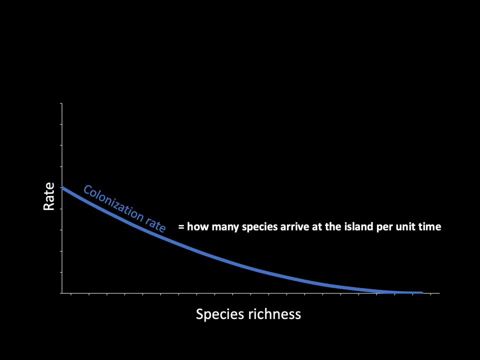 will represent a successful colonization event. However, as more and more species colonize the island, the colonization rate has to drop, representing that some individuals that disperse to the island are members of species that have already colonized it. The species that have colonized the island, though. 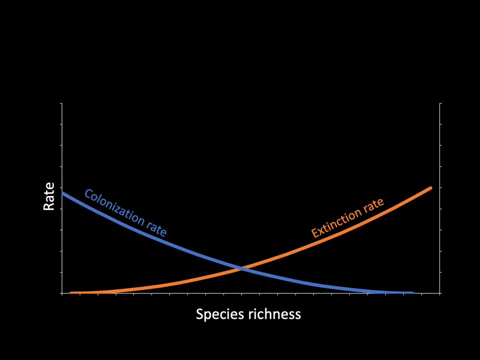 aren't guaranteed to occur on the island forever, And as more and more species colonize the island, there are more and more species that also can potentially go extinct on the island. In other words, when there are no species on the island, the extinction rate is zero. 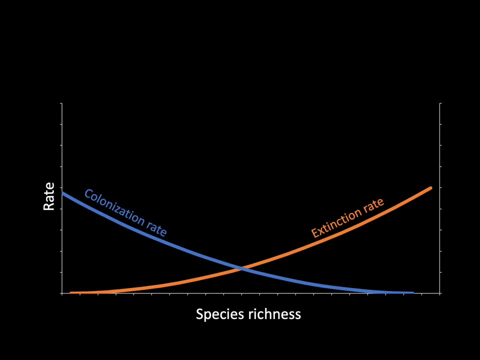 and when there are many species on an island, the extinction rate is higher, simply because there are more species that each potentially could go extinct. There's also another, more biological reason that we expect higher extinction rates on islands with more species, and that is because on these species-rich islands 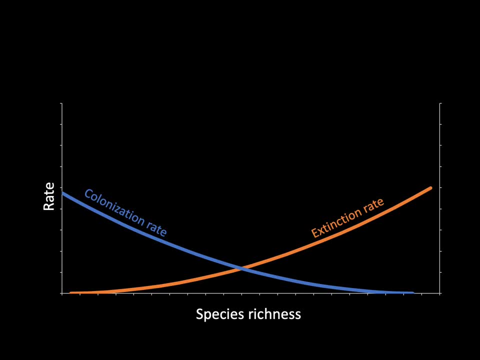 there's a greater potential for negative interactions between species, like competition, predation and parasitism, all of which can contribute to increasing the chance of a species being lost from the island. The balance, then, of colonizations and extinctions on any one island. 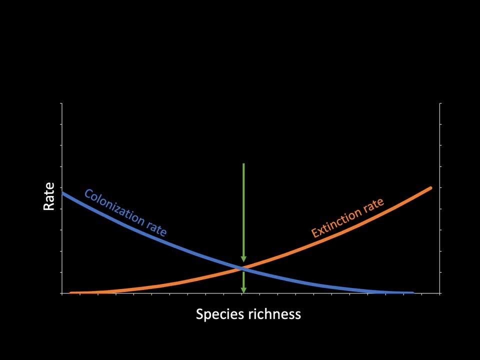 will determine the species richness of that island. This is why we speak of the equilibrium model. It means that the model is predicting the number of species that will exist on the island when colonization and extinction rates are balanced, in other words, when those rates are in equilibrium. 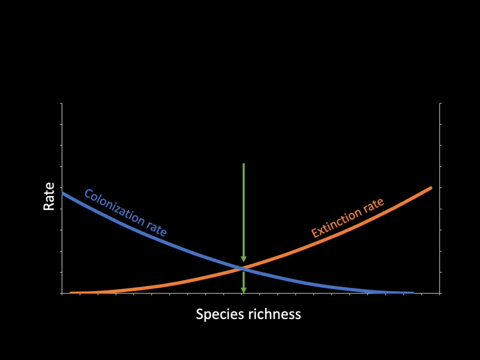 We see this on the graph as the point where the two curves intersect, In other words, where colonization and extinction balance each other out. So where it gets interesting now is when we adjust these curves for islands of different sizes or different levels of isolation. 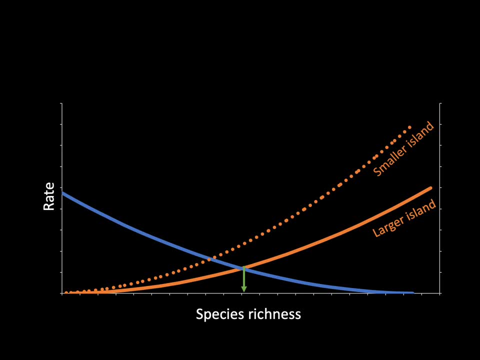 So let's think then: How does island size and isolation link with colonization and extinction? Well, bigger islands are more likely to be colonized, since they represent bigger targets for species to disperse to. They will also have lower extinction rates. 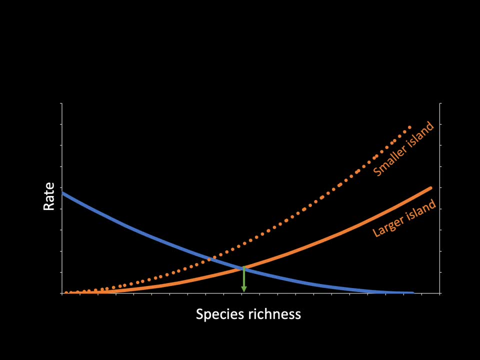 since species can have larger populations on bigger islands and therefore have lower probabilities of going extinct As a result. when we compare a larger island to a smaller island, we see that the intersection of the two curves occurs at a lower level of species richness. 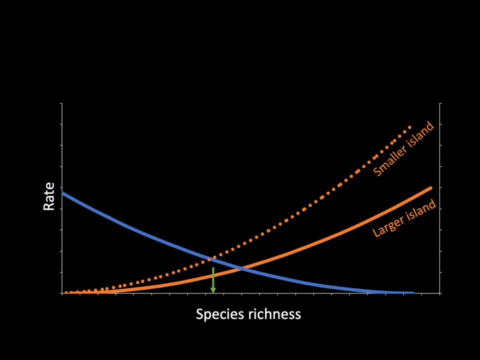 therefore predicting that smaller islands will have a lower equilibrium species richness than larger islands. Less isolated islands also have higher colonization rates and lower extinction rates, although for different reasons. When an island is less isolated, in other words closer to the mainland, it is more likely to be colonized by species. 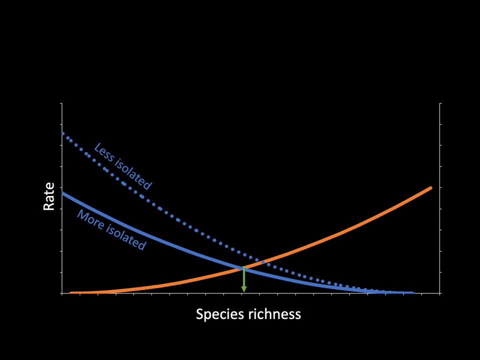 since species with good or with bad dispersal abilities have a chance to successfully arrive at the island. For isolated islands located far from the mainland, there will be a smaller number of species with the ability to disperse that far Less. isolated islands also have a lower extinction rate. 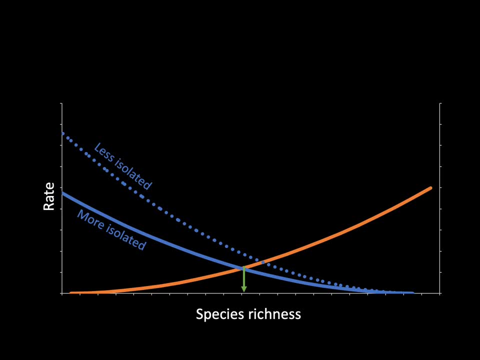 This is because an individual species will have a lower potential for extinction when there is more frequent dispersal by individuals of that species from the mainland to the island. In other words, a declining population on an island can be rescued by new individuals dispersing to that island from the mainland. 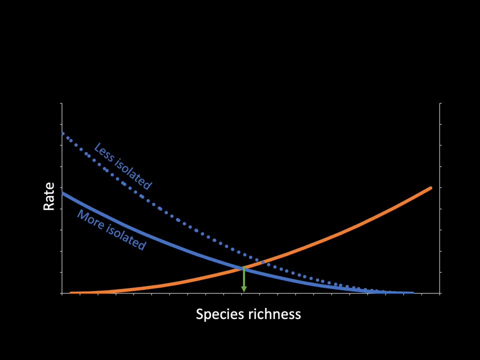 Therefore, when we compare a more isolated island to a less isolated island, we see that the intersection of the colonization and the extinction curves occurs at higher species richness values. Therefore, island biogeography predicts the highest species richness on large islands close to the mainland. 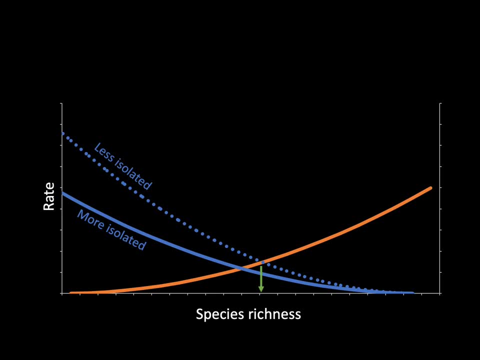 In other words, large islands that are not very isolated. In contrast, the lowest species richness would be expected on small and isolated islands, It's important to note. however, the theory only predicts the number of species on an island, not their identity. 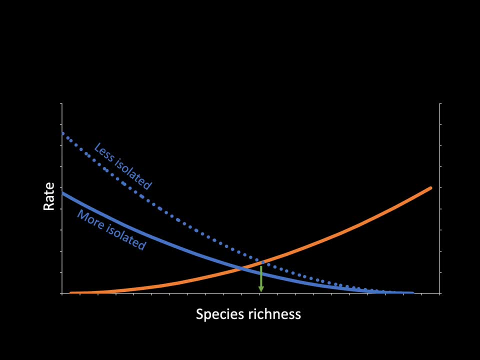 This is because it expects species composition to change through time. In other words, the theory predicts that through time there will be continuous extinctions and colonizations. So the species on an island would potentially change from time to time, But the balance of colonization and extinctions 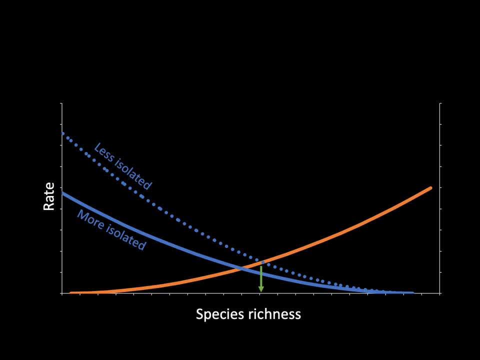 is expected to remain roughly the same, in other words, in equilibrium. As a result, species richness will be roughly similar. The changes in species composition that occur through time is what we call turnover, And it's important because it suggests that in a natural system, 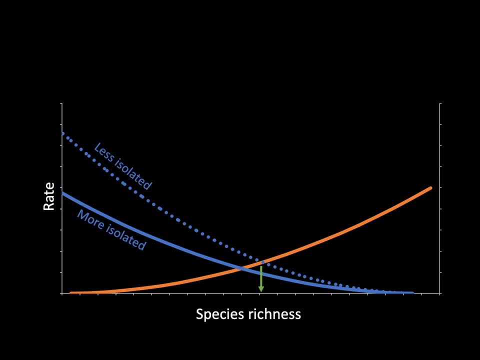 we expect to see change. In other words, even in a relatively short time period, there can be changes in which species occur on an island. So all of this sounds like a nice idea, but do you think that there are changes in species composition? 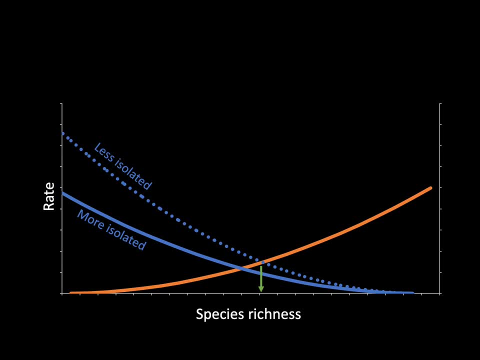 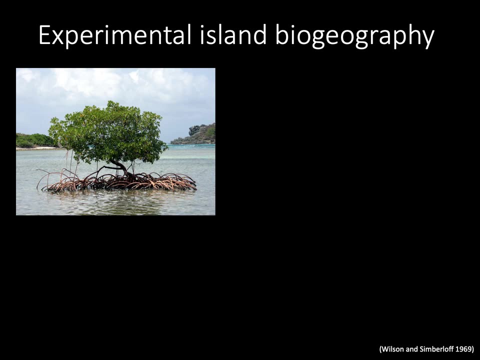 that occur on an island. Well, there are changes in species composition that occur on an island, but do our observations in the real world support it? In short, yes, There have been excellent studies that have tested the ideas of island biogeography. 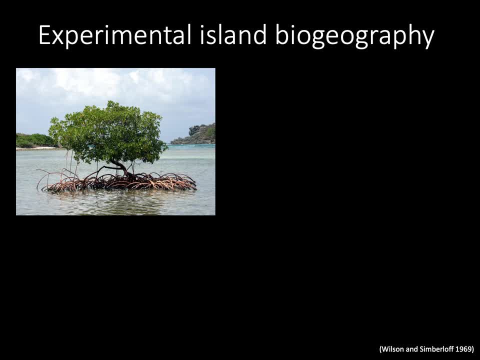 with many providing support for the predictions of the theory, For example, in a very bold experiment, Dan Simbaloff, who was a student of EO Wilson, who, of course, was one of the two ecologists who developed this idea initially- 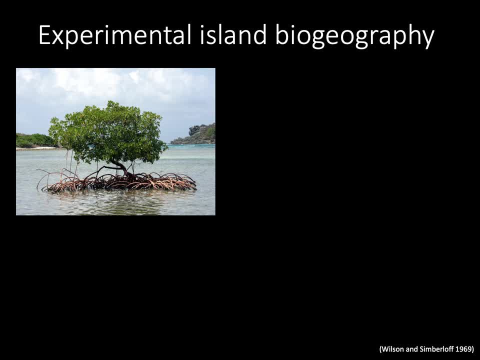 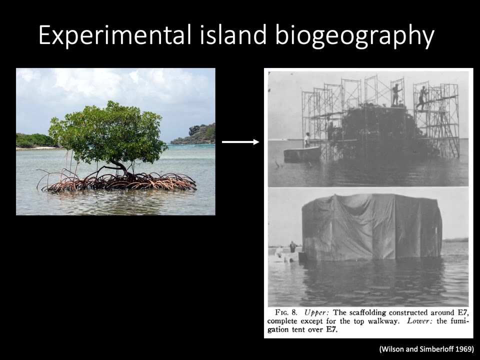 he looked at the existence of the invertebrates living on small mangrove islands just like this one in the image here. After documenting the fauna of each of six of these small mangrove islands off the coast of Florida, he wrapped them up in big. 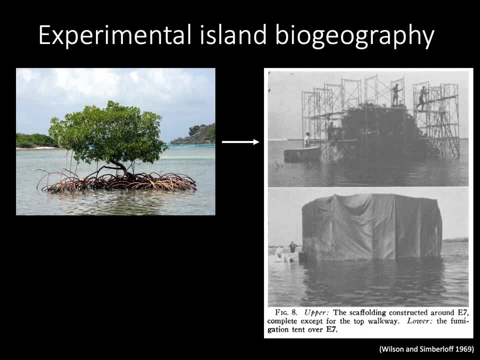 plastic sheets and fumigated them, killing entirely all the insects and other invertebrates in the tiny islands. He then monitored the animal species colonizing the islands for a year and found that the invertebrates were colonized by roughly the same number. 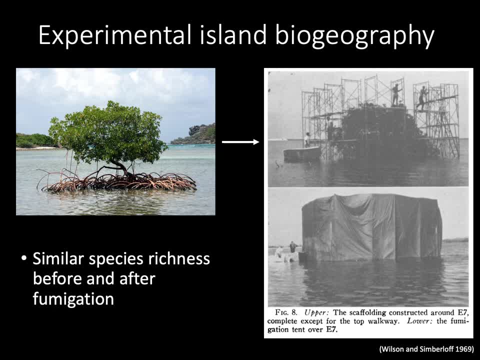 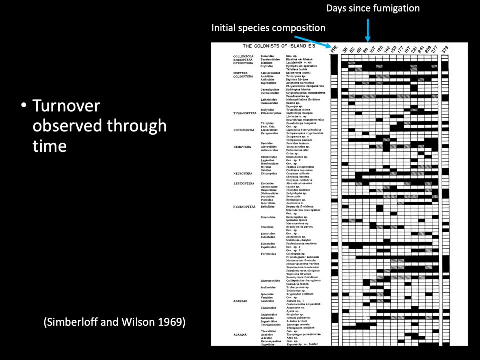 of species after one year, as that had occurred on the islands before they were fumigated. Therefore, the species richness on the islands returned to roughly the same equilibrium richness as the islands were recolonized after fumigation. He also found turnover in the 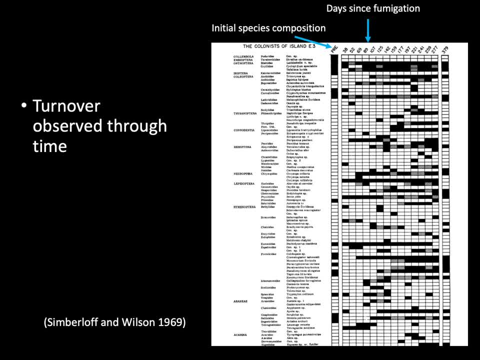 species composition occurring through time. You can see this in this extract from his results. Now, in this table, each row represents a different species and each column represents a different time at which he recorded the species on this specific island. The first column shows: 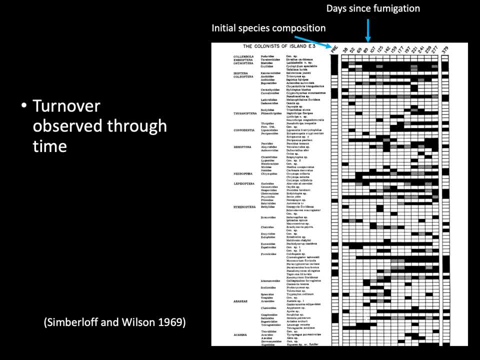 the number of species that were there roughly after one year of recolonization. after fumigation, Filled cells represent when a species was recorded and the empty cells represent when a species wasn't found. What is really clear here is that the number of 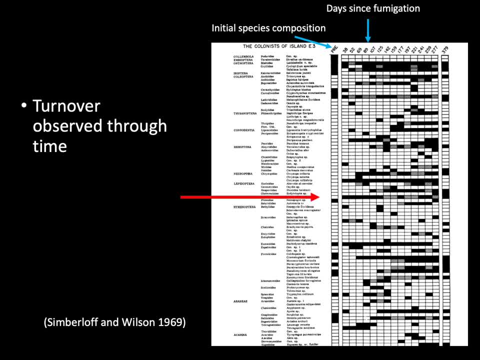 species that were recorded in the initial pre-fumigation survey was blank, So it wasn't present on the island before fumigation. What you, though, do see is immediately after fumigation it colonized the island. We can see a different. 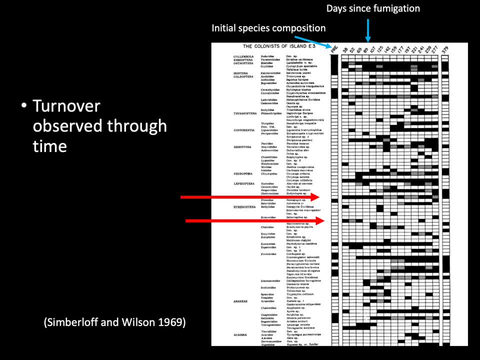 pattern for this parasitic wasp. This species was also absent before fumigation. Then it dispersed to the island. You can see there are a few cells that are filled, but it did not persist on the island before fumigation colonized. 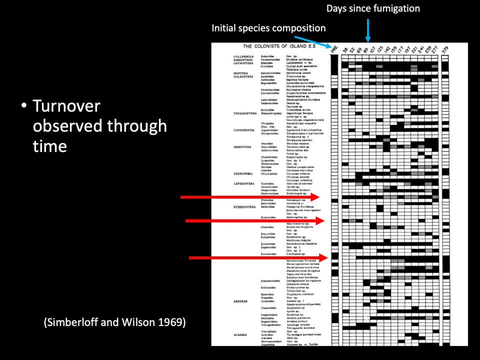 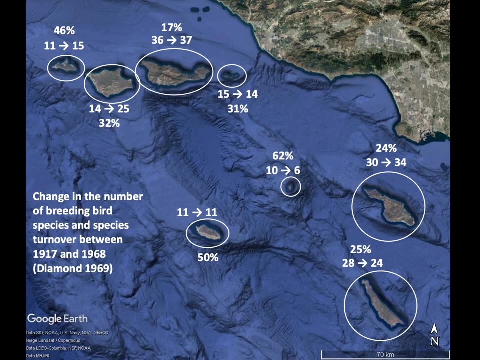 the island after two months and then didn't go extinct on the island for the rest of the year. So this then nicely illustrates island biogeography theory's impact on the species of the small islands offshore of California and found that compared 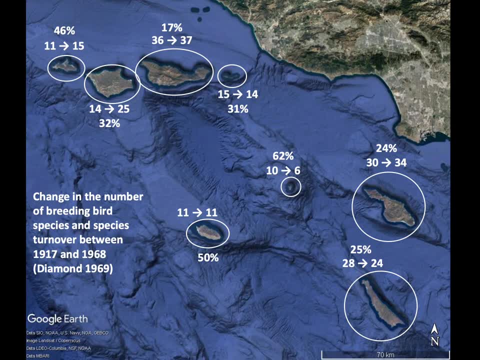 to an earlier survey conducted 51 years previously, the number of species had only changed slightly, from 17 to 62 percent. In other words, colonization and extinction events had altered which species occur on those islands, with some big changes in species composition. OK. 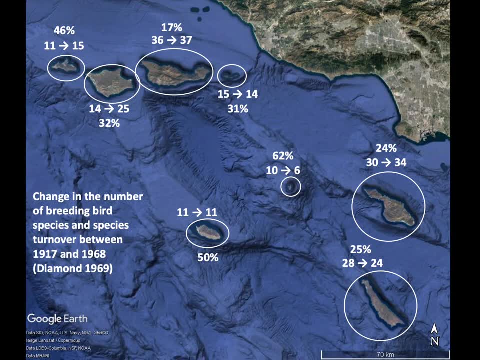 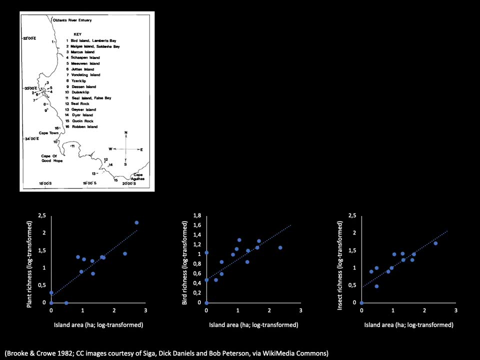 but what are the results of this study? Here we also have good evidence from multiple studies that support the theory of island biogeography. Let's come back to South Africa now, where we have three taxa In each of these three graphs. 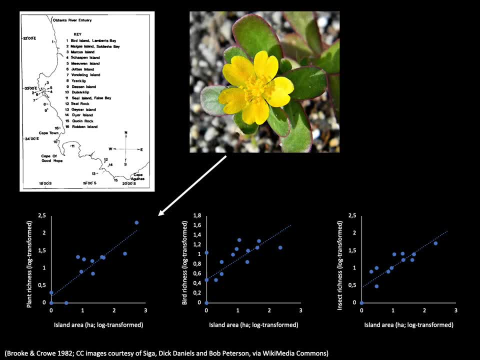 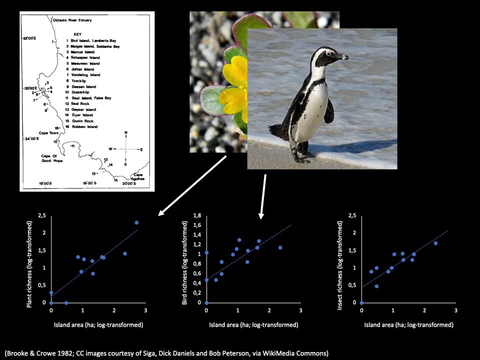 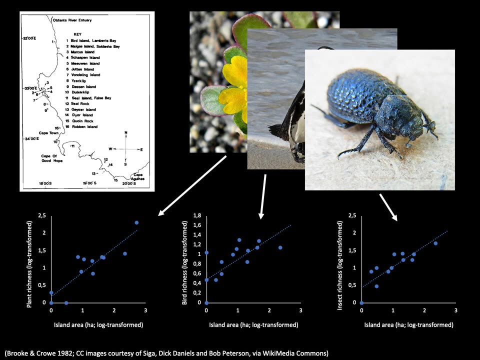 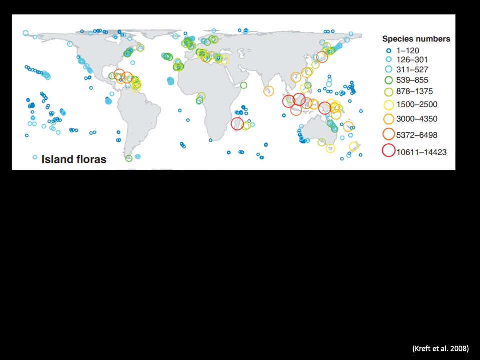 on the X axis you can see we have island area and on the Y axis we have different species. We can also look at islands globally. Holger Kreft and colleagues recently examined the plant richness on 488 islands globally In this: 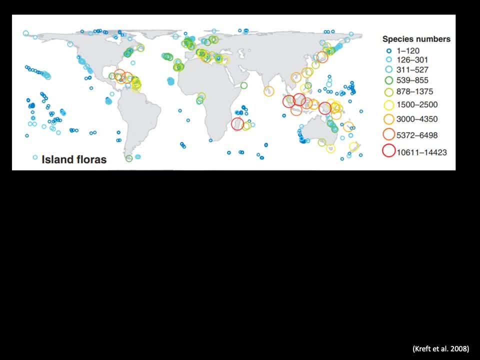 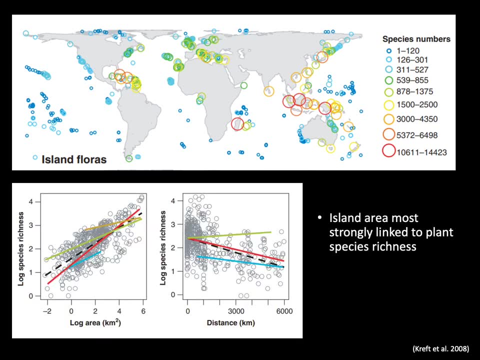 image. here you can see how much variation there is in these islands. They analyzed the data in a number of ways and found that area was the best predictor of plant species richness on these islands, followed in by the island biogeography theory. 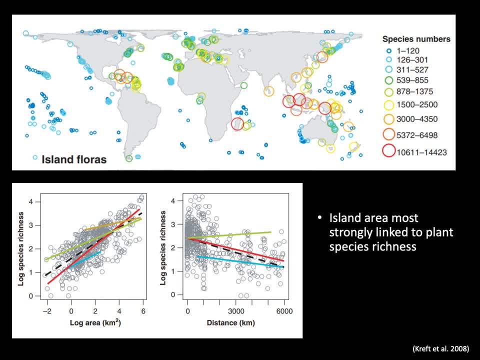 In the graph on the right-hand side we see a negative relationship between distance and species richness. Here distance is their measure of isolation. In other words, the island biogeography theory is based on the island biogeography theory In the. 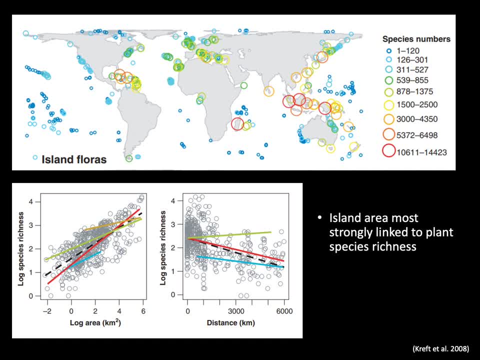 graph on the right-hand side, you can see that the island biogeography theory represents the overall pattern across the island. In the graph on the right-hand side, you can see that the island biogeography theory is based on the island biogeography. 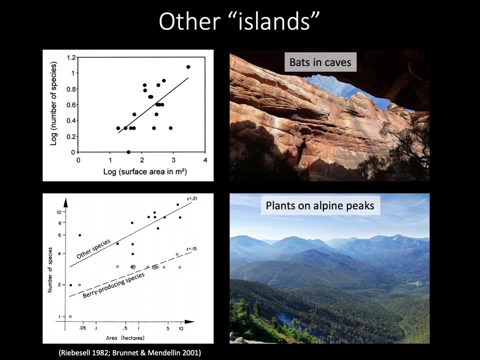 theory. In the graph on the right-hand side you can see that the island biogeography theory can be applied to any habitat that acts like an island. In other words, any patch of habitat separated from other caves is considered a habitat island. 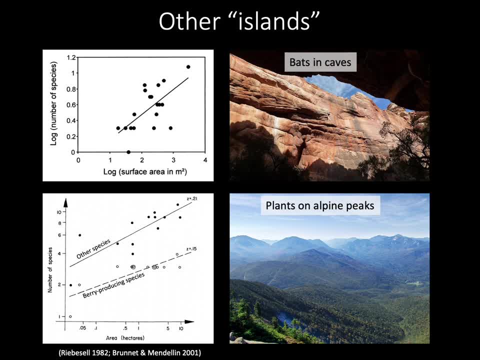 So the ideas of island biogeography can be useful for patchy environments like, for example, caves which are separated from other caves by areas that are very different habitats. The island biogeography theory can be applied to all types of habitat. 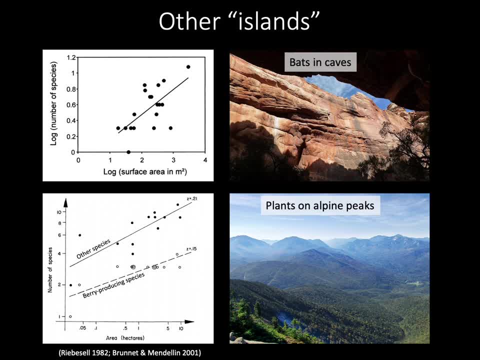 and for some groups of species. For example, studies have shown that groups of isolated caves and high level caves are much larger than those in the first graph. The graph shows how the size of alpine mountain area gets bigger, and so the number of plant. 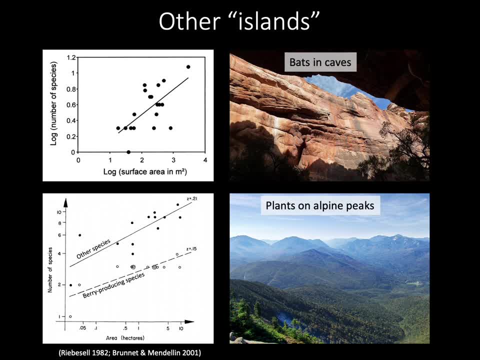 species increases. In this graph we've got two lines. This represents berry producing plant species, which are, of course, expected to have good dispersal by animals, as well as non-berry producing species, which are expected to have poorer dispersal. And 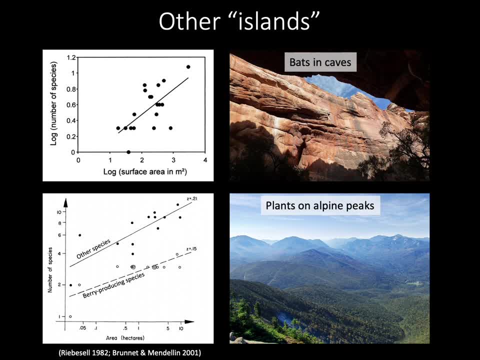 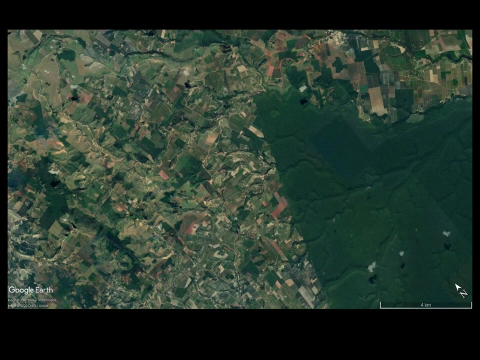 in the graph we can see that the size of alpine mountain area is much larger than the size of alpine mountain area. In this graph we can see that the size of alpine mountain area is much larger than the size of alpine mountain area. 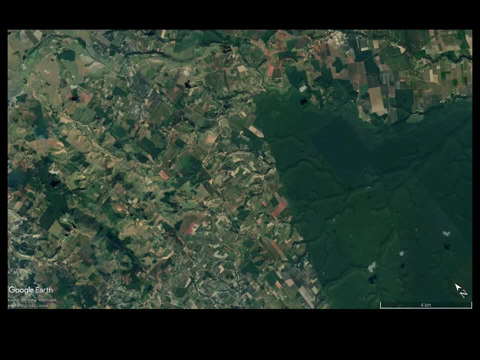 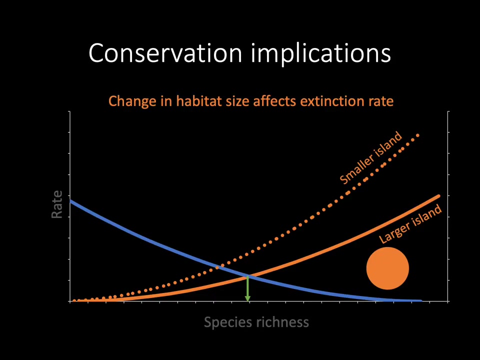 In this graph we can see the size of alpine mountain area. There's a clear mainland area of forest on the right and the little islands of remaining natural forest occur all around that mainland. I think there are two key points here: that island biogeography. 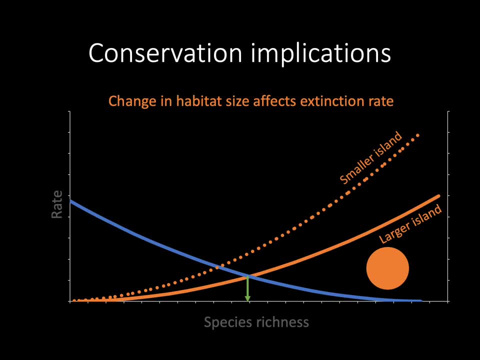 theory can tell us about this. This results from smaller islands having lower colonization rates and higher extinction rates. As an example here: as we decrease habitat patch size, we increase extinction rate and lower colonization of habitat. We'd expect a similar effect from lower colonization.